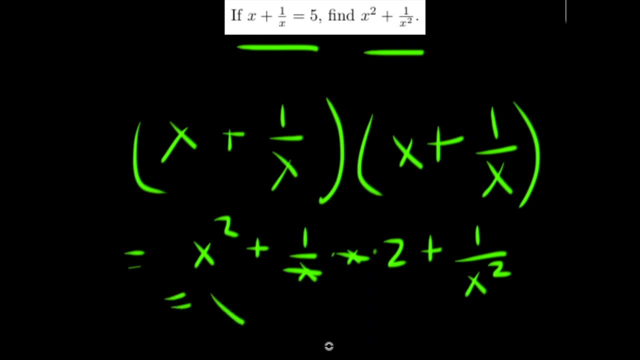 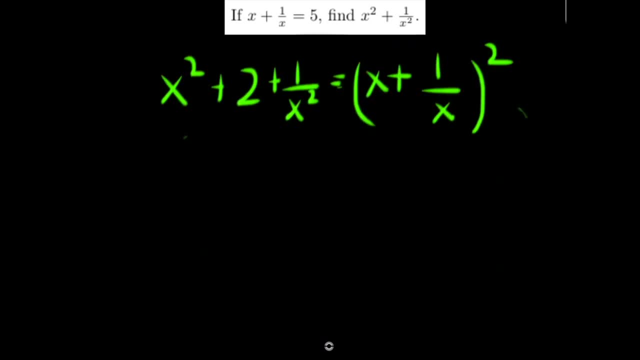 The x's will cancel and then you're left with x squared plus 2 plus 1 over x squared. So I just rewrote that up here We have x squared plus 2 plus 1 over x squared is equal to x plus 1 over x, the whole thing squared. 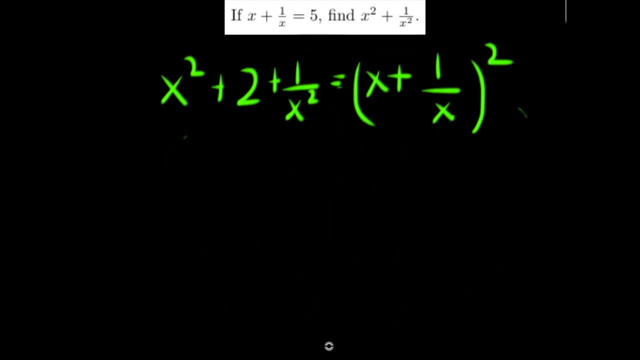 And it's given to us that x plus 1 over x is equal to 5.. So let's go back to the original equation, Go ahead and plug that. in Rewriting this, x squared plus 2 plus 1 over x squared is equal to. we're substituting in 5,, 5 squared. 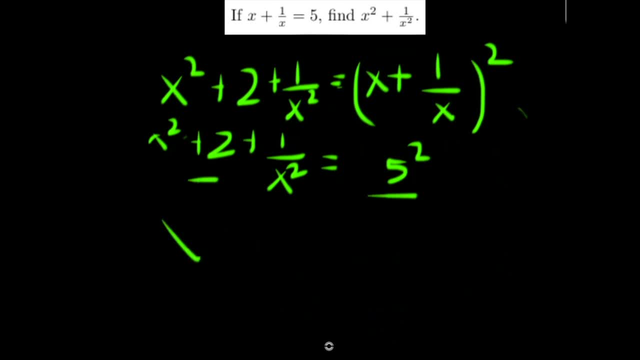 And, as you can see from here, it's just simple subtraction: x squared plus 1 over x squared is equal to 23. And that's our answer for this problem. These types of manipulations also work for higher powers of x. Here's another problem. 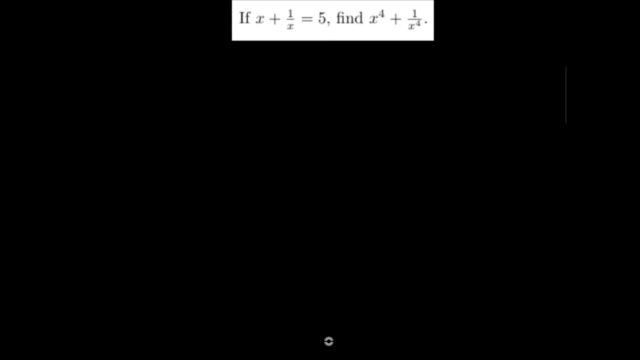 If x plus 1 over x equals 5, find x to the 4th plus 1 over x to the 4th. So we have to see again how do we go from a power of x to the 1st to x to the 4th. 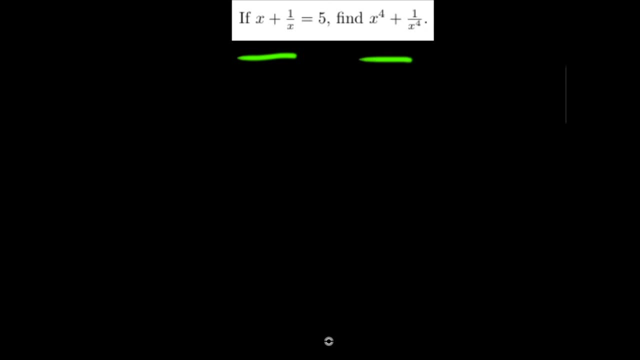 And the easiest way to do that is obviously just raise that to the 4th power. But what does raising something to the 4th power really mean? Saying something is x to the 4th is the same thing as saying something squared squared. 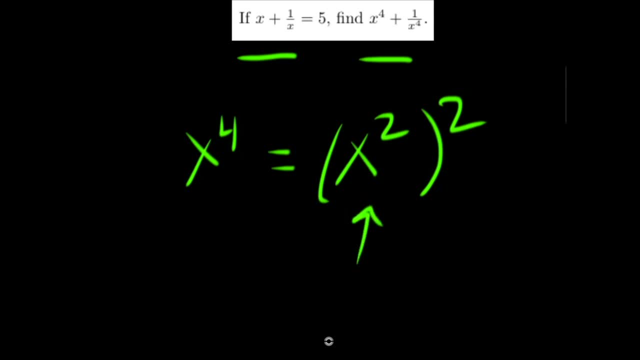 So the first step of this problem would be to find what x squared plus 1 over x squared would be, and then squaring that to get x to the 4th. So we start our problem in the same way, We do: x plus 1 over x equals 5, and we square the whole thing. 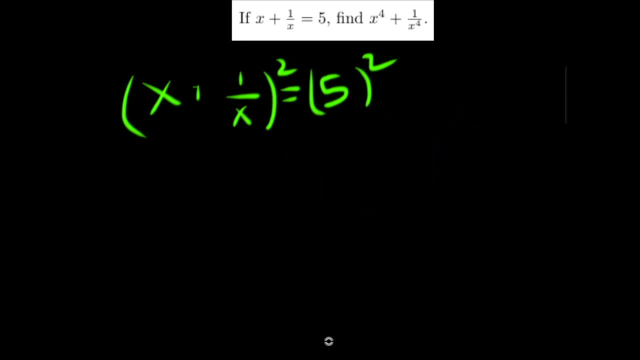 And we square both sides And you get x squared plus 2 plus 1 over x squared equals 25.. And you get x squared plus 1 over x squared equals 23.. This is exactly what we did before. I'm just copying that over. 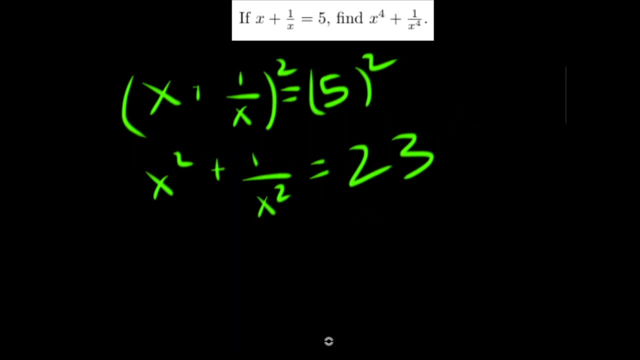 So we do the exact same thing. We do x squared plus 1 over x squared. We square that whole thing and then we square the 23 as well. So we square this, square this. You're left with x to the 4th plus 2 plus 1 over x to the 4th is equal to 23 squared, which is 529.. 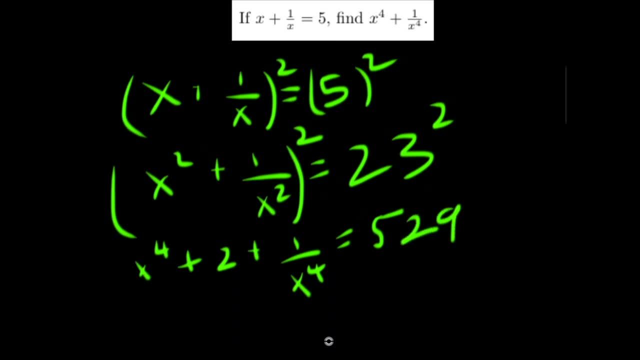